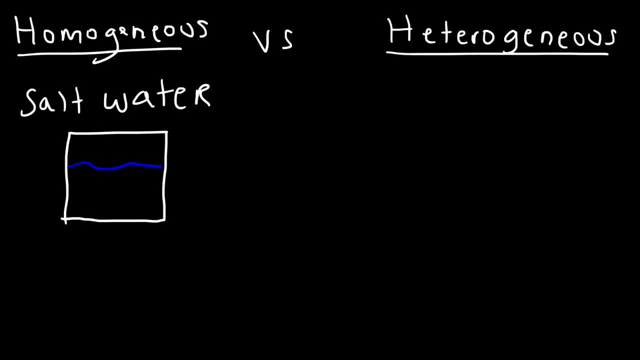 or more pure substances. Oil and water do not mix. You can visibly see two distinct parts Now. water is more dense than oil, so the water layer is going to be below it. The lighter oil layer is going to be above it. So because oil and water do not mix, 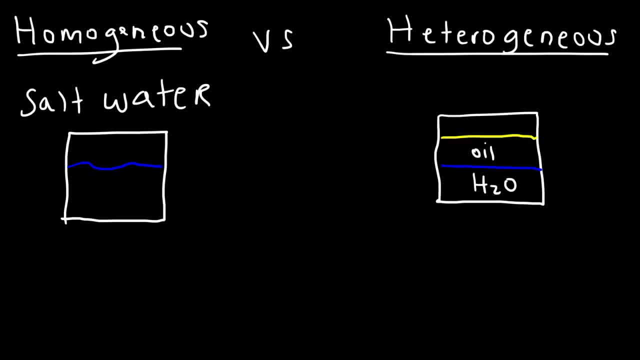 you can see, it's a heterogeneous mixture. You can see the two visible parts. Now what about brass? Is brass a homogeneous mixture or is it a heterogeneous mixture? Brass is a homogenous mixture. Brass is an alloy. It's a solid solution of zinc. 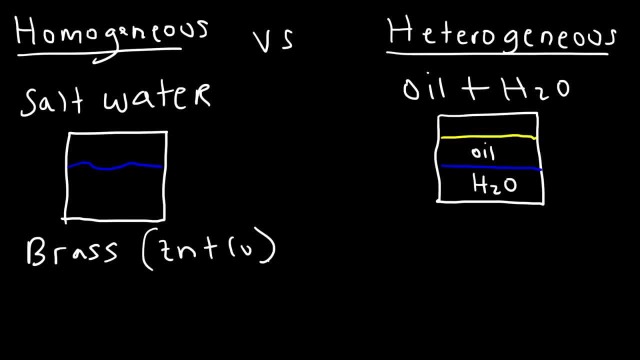 and copper, And these atoms are distributed uniformly throughout the material. So most alloys tend to be homogeneous mixtures. Their composition tends to be uniform. Now what about sand and water? Is that a homogeneous mixture or is that a heterogeneous mixture? Sand and water is a heterogeneous 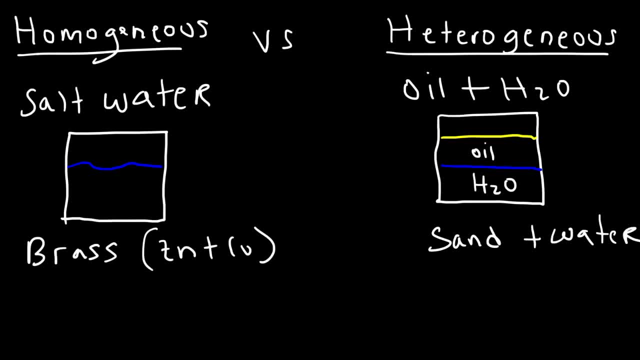 mixture. You can clearly see two distinguishable parts. Salt dissolves well in water, so basically it's. you don't see the two distinguishable parts. But sand- sand doesn't dissolve well in water. If you put sand in water. 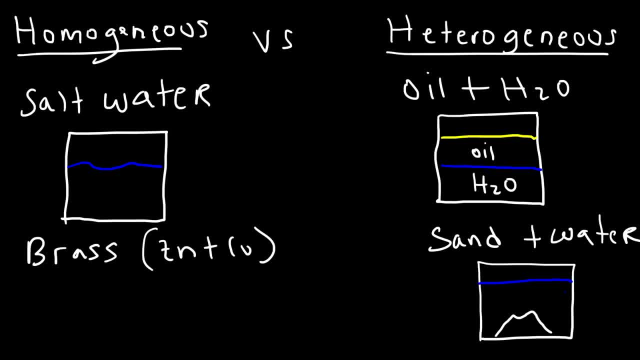 the sand will just fall to the bottom and you could see the sand in the water. You could see the two distinguishable parts. So sand water or sand plus water, that's a heterogeneous mixture. Now what about air? Is air a homogeneous mixture or a heterogeneous mixture? 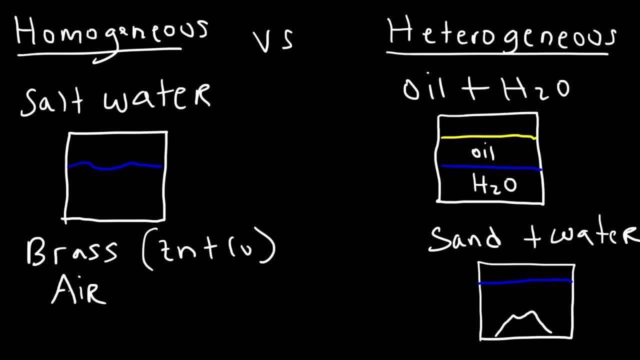 Air is a homogeneous mixture. You don't see visible parts in air. You don't see red air or blue air. It's just. it's just air. It's uniform in composition. Air contains nitrogen gas, oxygen gas, argon gas and oxygen gas.